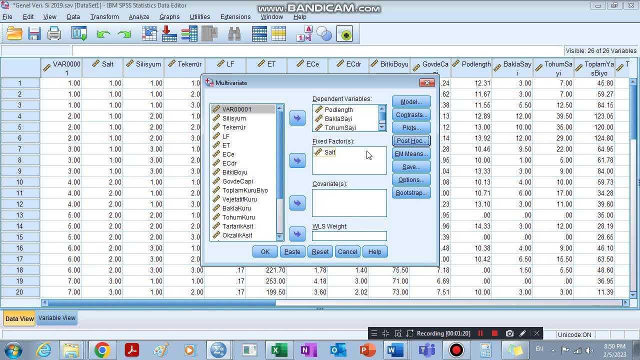 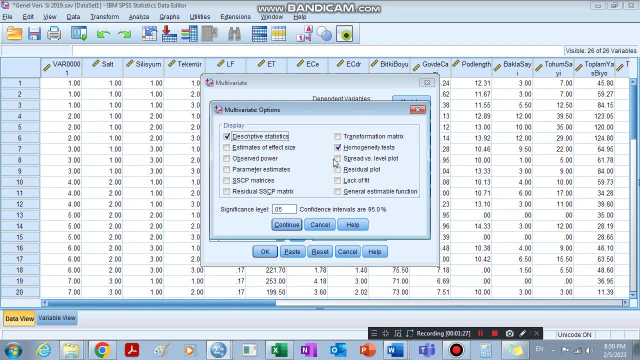 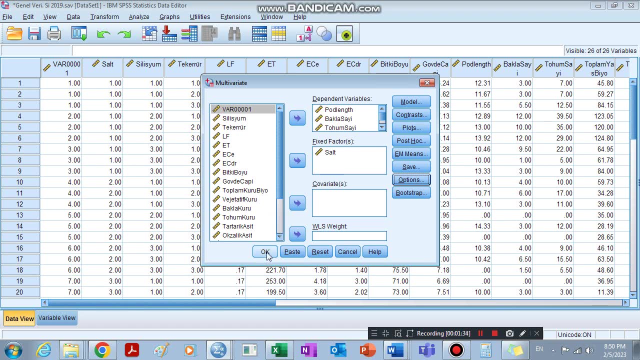 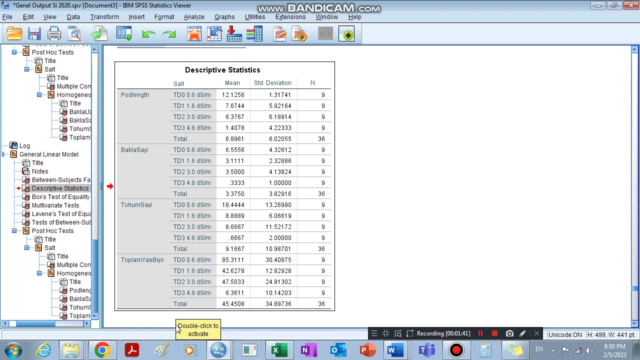 Duncan. then you click OK, you go to the option menu and you highlights descriptive styles and homogeneity tests. then you click on continue, then you click on ok, then when you click on ok, you will get this result. after analysis, this indicates that both potlings, our dependent variable, is affected significantly affected by salt. 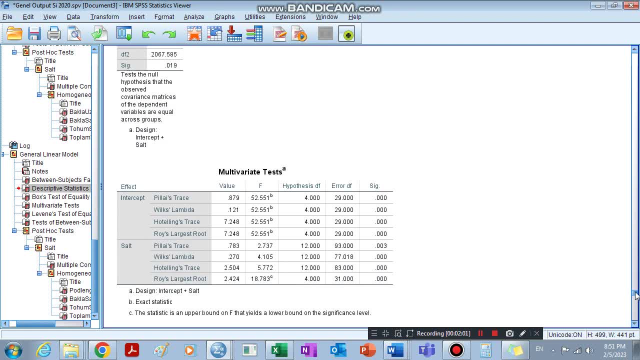 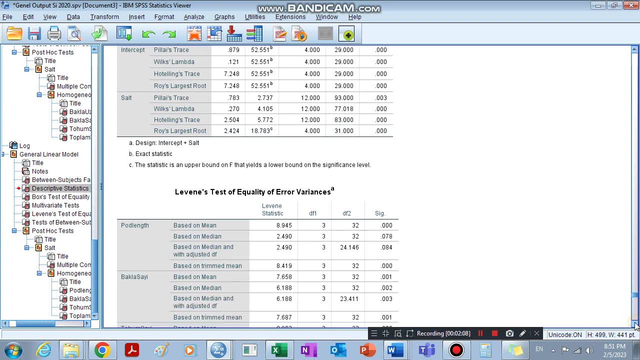 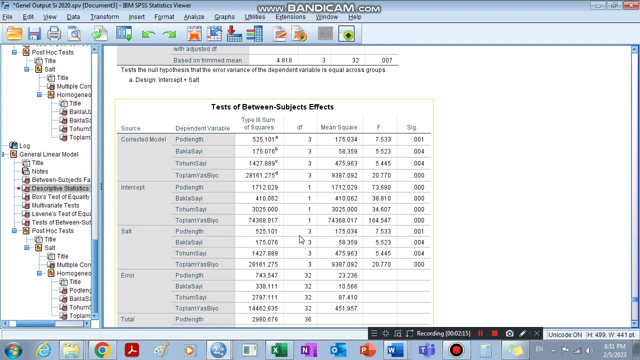 different salt levels to see how it is significantly affected. we can check it here. we can check it here. and salt: it is significantly affected. the pod language is our dependent variable. here is a fixed, significantly affected by salt. different salt labels. how do we know it is significantly affected? because it is, it's a factor if value is less than 0.05. 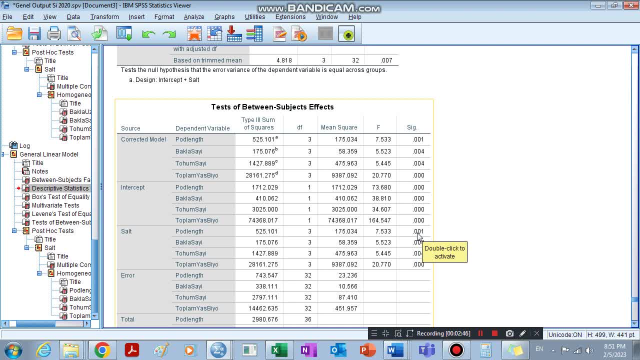 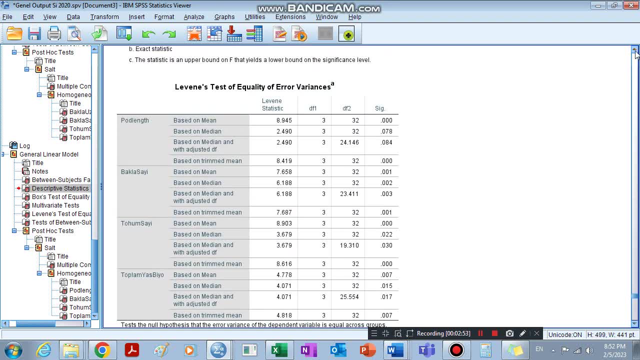 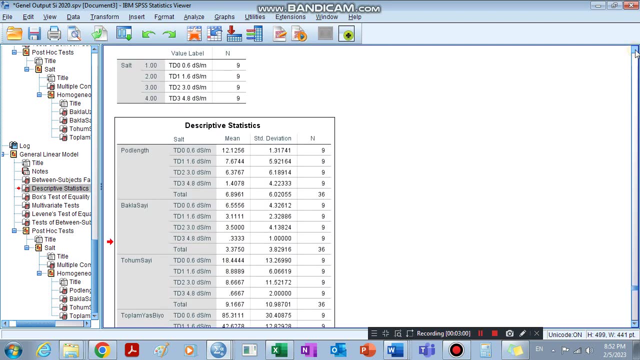 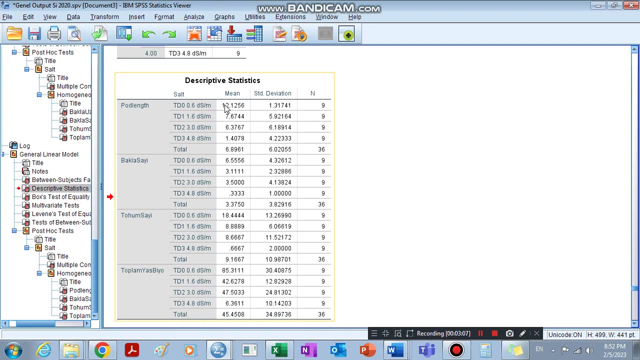 which is at five percent significant level. so it's significant. so how do we transfer the values, which values are taken, are taken, to analyze, to interpret our result? these are the values we are going to take. this are the values. so to take the values we can just. 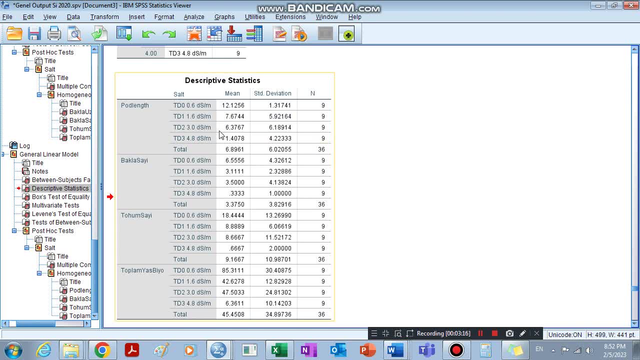 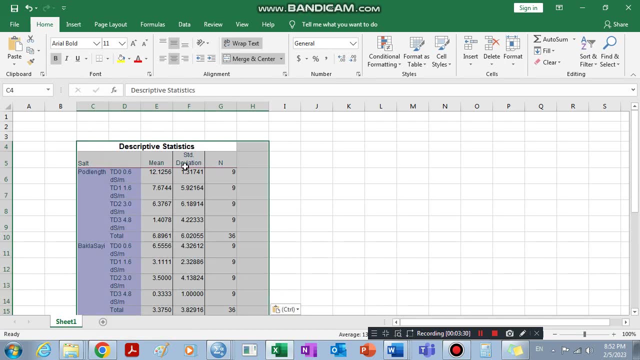 copy it copy. we can first take it to our Excel page, Excel worksheets page, so that we can take it to our our work documents. then we can interpret it, we can, you know, explain it. then we can take each numbers by copy and paste to our document here. 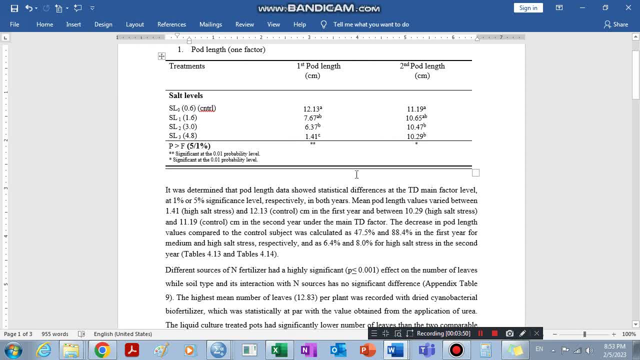 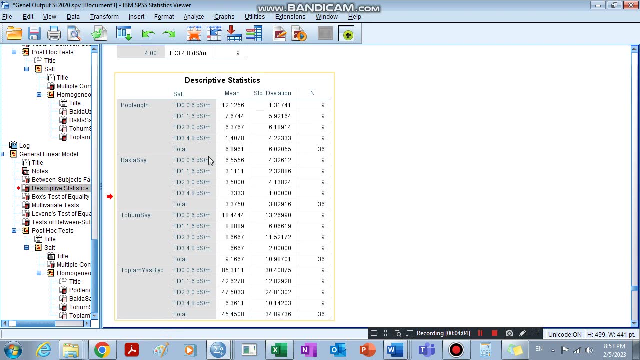 then interpret it. I took the documents, the values here already. I took it from here as I to either showed you from descriptive statistics table from here, after analyze, analyzing from our output s pcs output, we find descriptive statistics table. that's where we are taking our values, the values of the analysis. 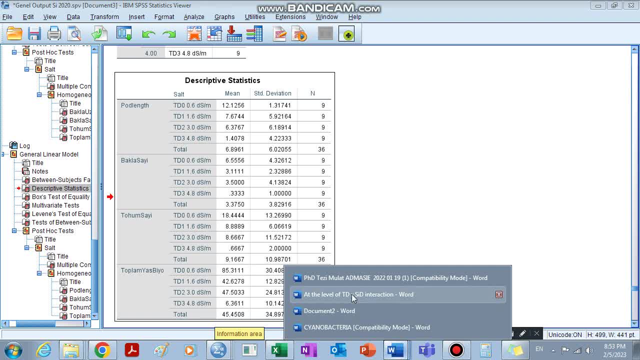 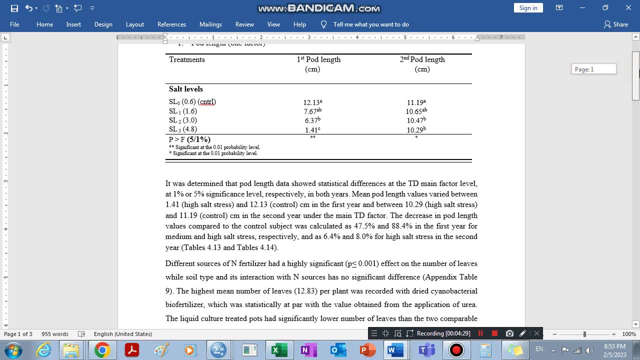 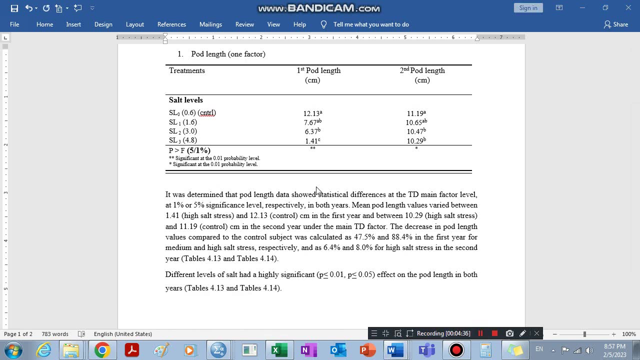 result from then, after taking it, we can interpret it in such a way that this is an example, that's i'm going, i'm going to show you how to interpret the result. so here we can say that it was determined that pod links, our dependent variable, showed that positive pod, the data or the analysis, 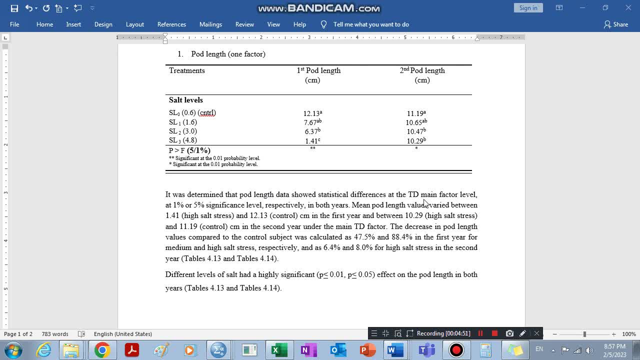 result. another result showed that statistical difference at the salt level main factor level at one and five significant level respectively in both years. it's significant statistically, uh, significantly significant, or we can say that different levels, levels of that had a signal highly significant at one percent probability level and five respectively in different years. 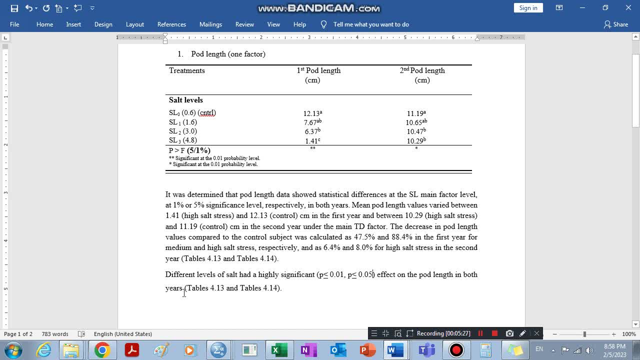 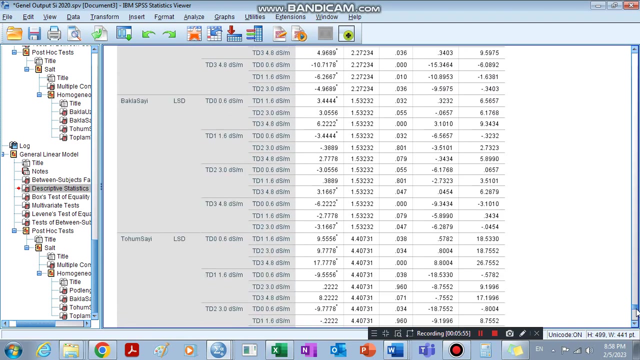 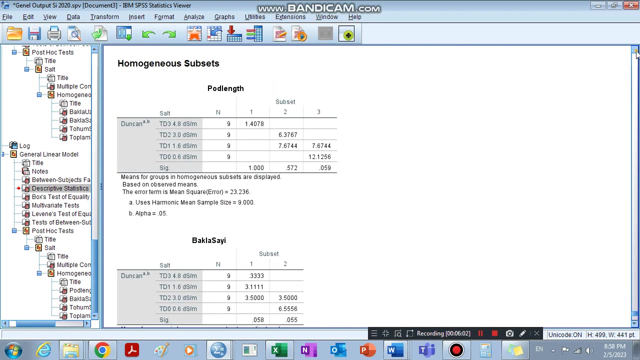 effect on pod links in both years. we can say it in different ways, it doesn't matter. the most important thing is that it has to be explanatory, which means it is significantly affected. this letters, where do we find them? we can find them from here. from here, when you go down to the, the end of the page. you can find it here. from still, from the. 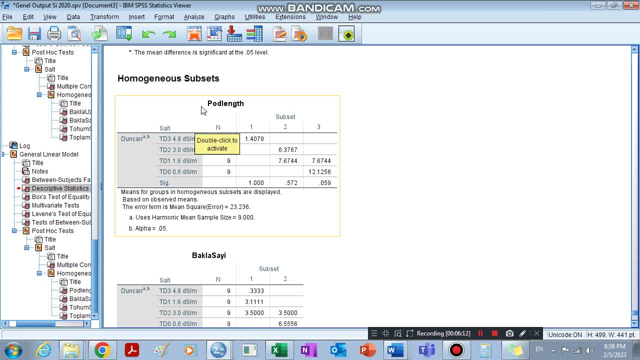 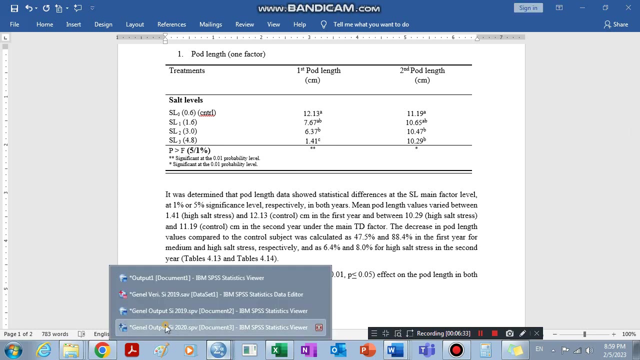 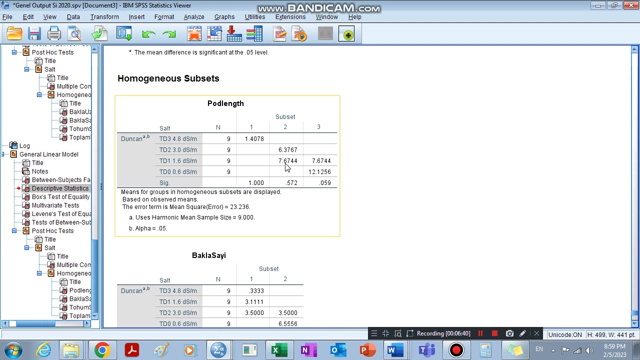 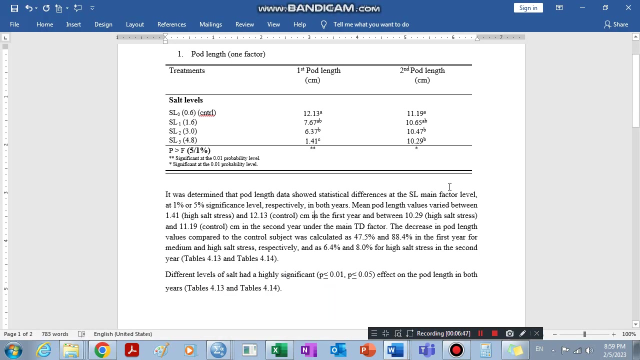 page on the uh species outpost page, pod links. this is here. is you how you are going to label the, the numbers, by different letters? for example, you can label this one a, which means a, 12.13- 12.13 it's approximately uh. this one, 7.67, is a, b, which is already written it here, a as a b and the other one: 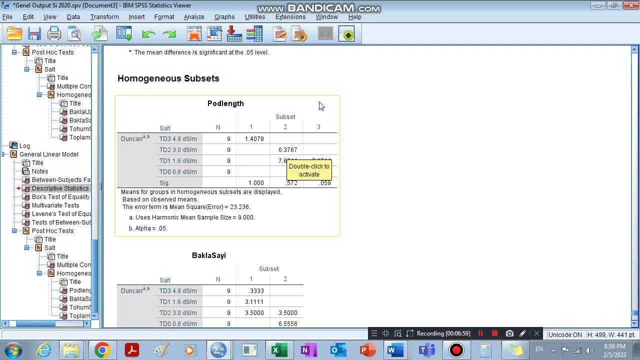 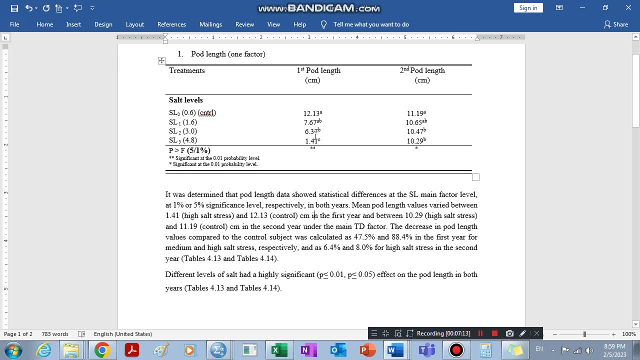 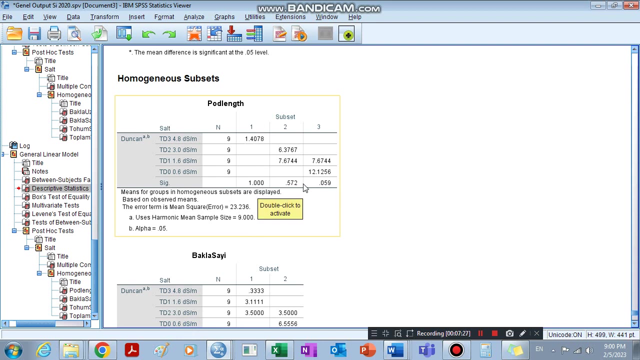 this one is b because this one, this color man is, is supposed to be a and this one is b. this 6.38, almost, is b, 6.37 is b and the last one, 1.41, is c. this one is c a, b. c a is the, the biggest that i in the 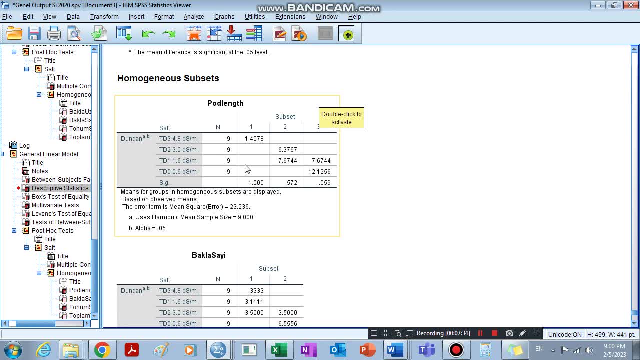 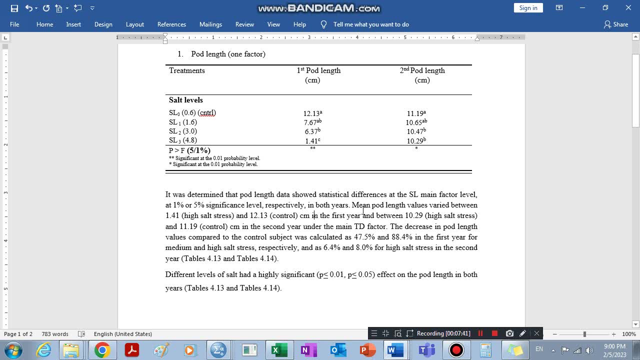 you know the highest number, then b, c. this is how we uh write the numbers, write the levels. then we can uh go ahead and further explain that mean pod length value varies, varied between one point four one, between one point four one. highest salt stress: we can you know further explain like this: and between 1.41 and 1, 12.13. 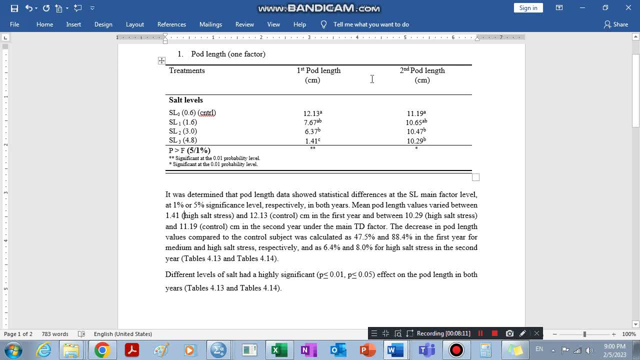 12.13. we can, you know, explain every detail of the table which is already here, and we can also calculate the percentage on which it decreases because of the high salt stress. as the salt level increases, its value, the puddlings of the plant decreases because of the salt stress. so in to